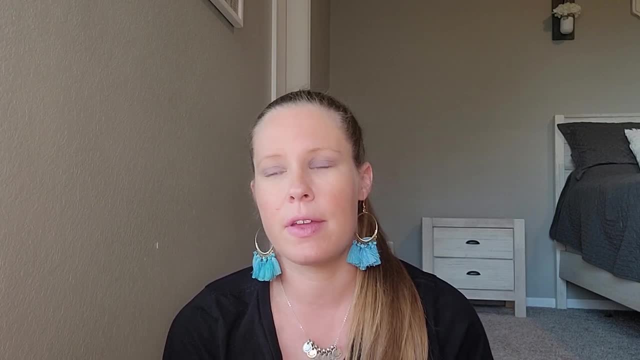 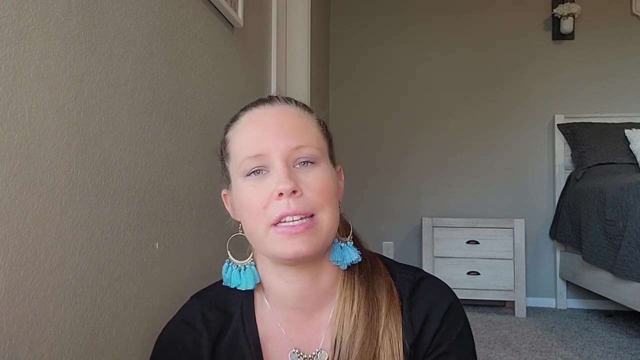 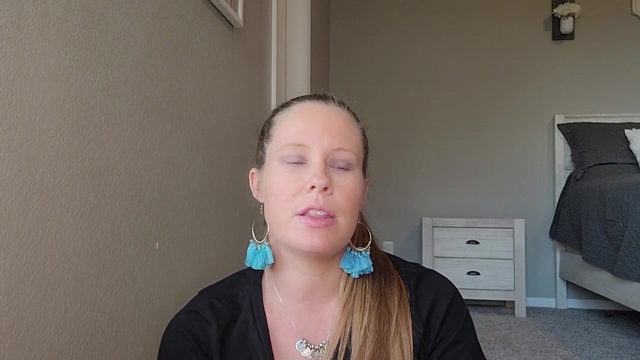 little bit different, because she was kind of getting burnt out of just all the extra stuff that is included in the lessons, And so language arts is one of those ones that I've had trouble with. I knew from the very beginning of homeschooling what my kids do best with, And really The 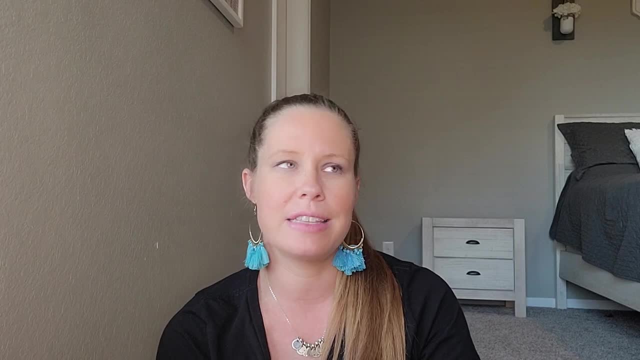 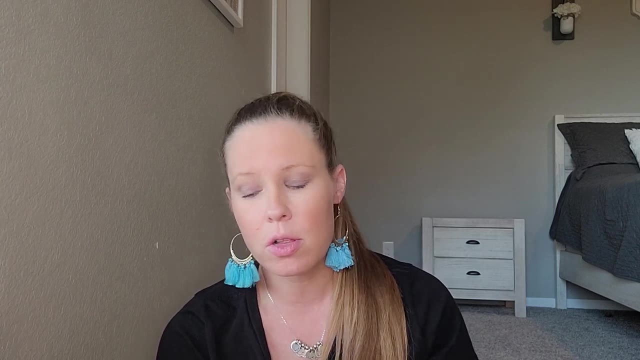 Good and the Beautiful. I love their language arts program But, like I said, sixth grade, I knew I didn't want to do. We haven't gotten to that point where they have redone that particular level yet, And so it's still like the very lengthy lessons, And I just knew. 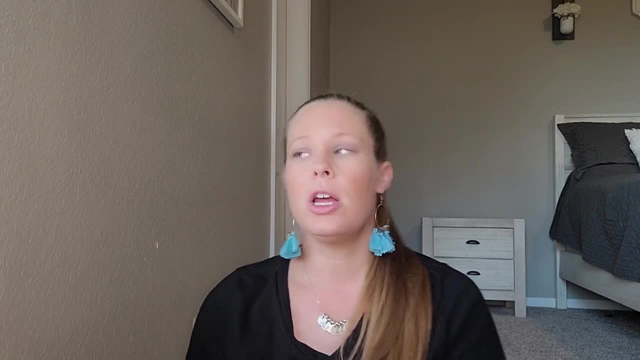 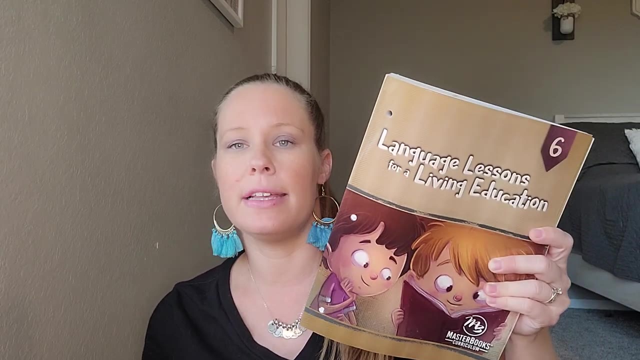 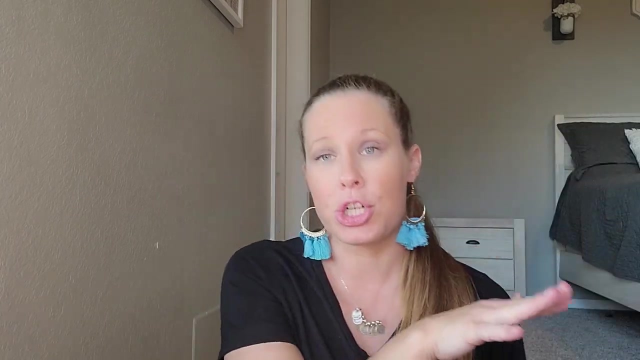 I knew it wasn't going to work for her, So I said, nope, we got to find something different for this coming school year. And so I ended up getting was master books, the level six language lessons for living education. Now I'm not sure if I will continue master books after this or if I'm going to 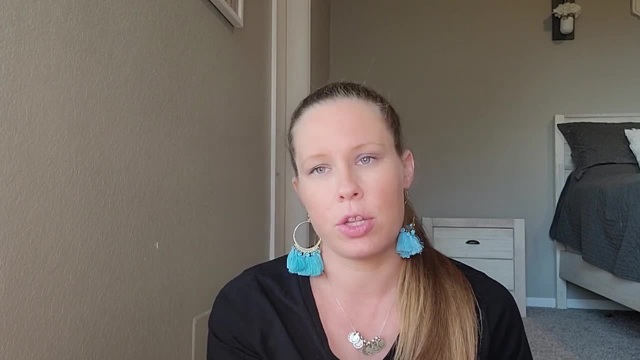 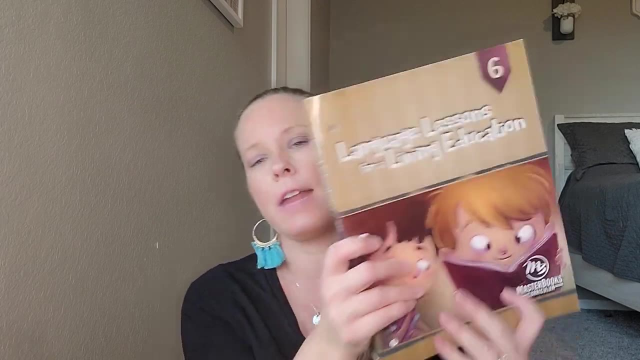 go back to the go to the Good and the Beautiful. I will probably go back to the Good and the Beautiful, But I knew for sure for a level six that I needed something different, So I wanted to just kind of do a flip through with you on this. 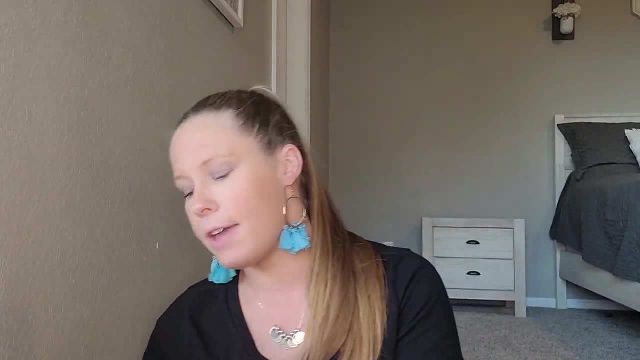 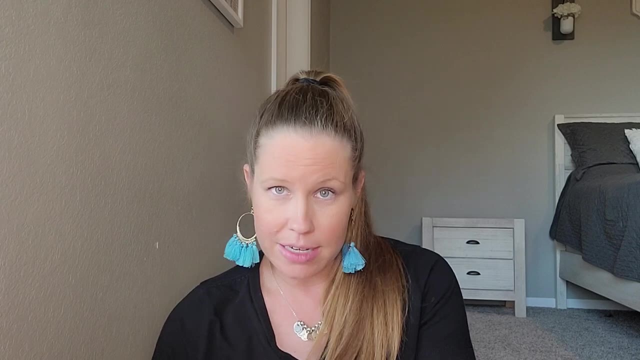 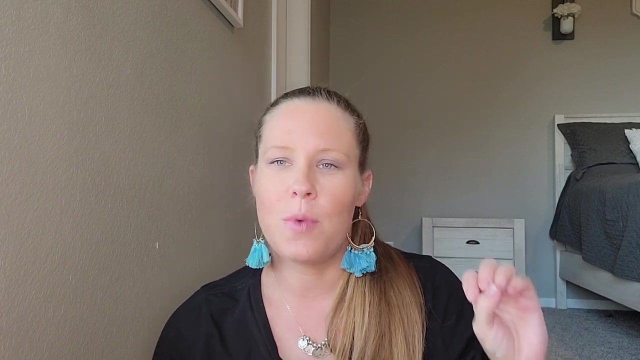 00.00.. 00.00.. 00.00.. I feel like there are some things that she already will know. I am okay with that. Okay, Let me make that clear. I am okay with that because the worst thing is to have a child. that. 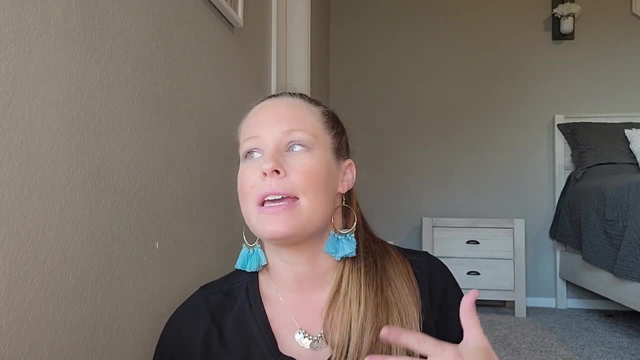 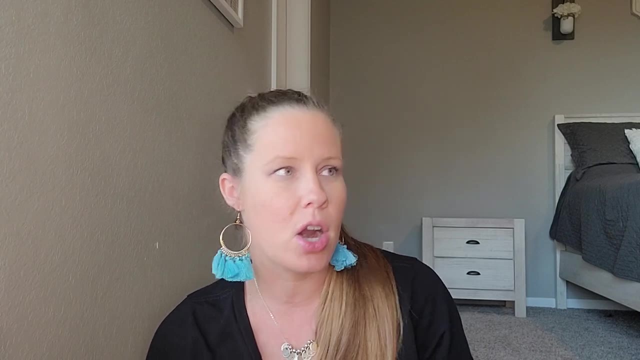 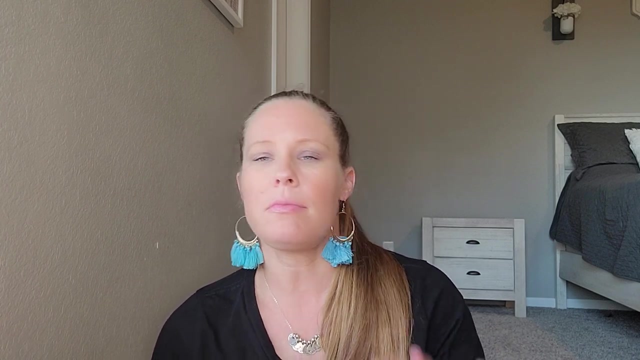 is struggling and you are trying to push them because maybe you don't realize that there's that gap in between curriculum pieces, that that was missed somewhere, or you feel like they should know it but they're having trouble grasping it, or for whatever reason. that is the worst and 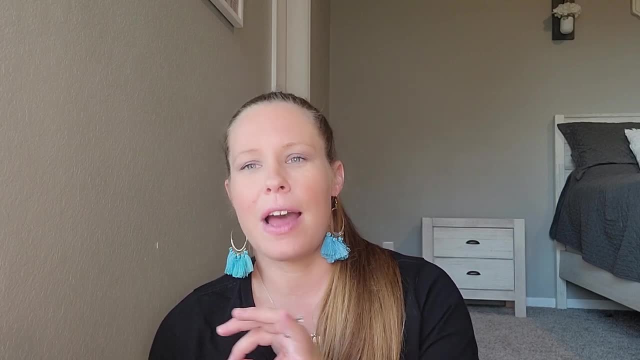 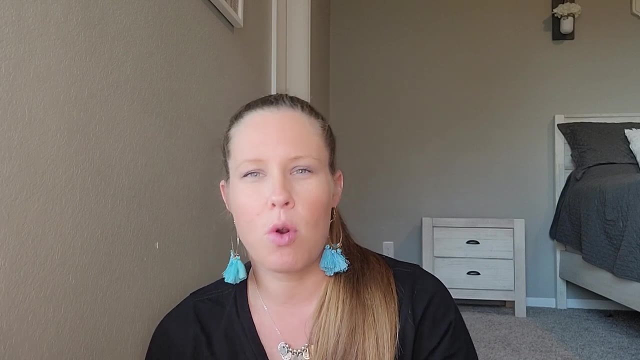 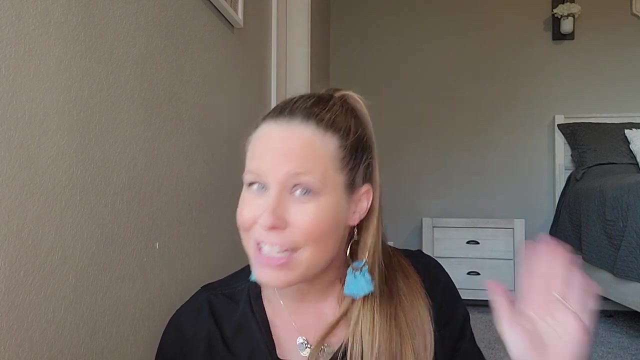 having to deal with, I'm telling you, And so I am okay with them doing things as a refresher at the beginning or realizing that, Hey, this curriculum has some things that I already know. Great, Great, Let's do them and keep going. Okay, Um, so I am okay with that. 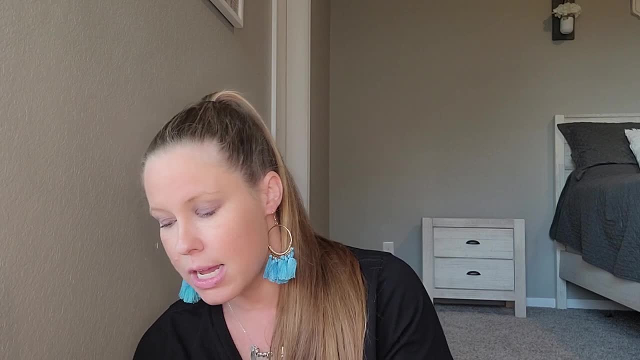 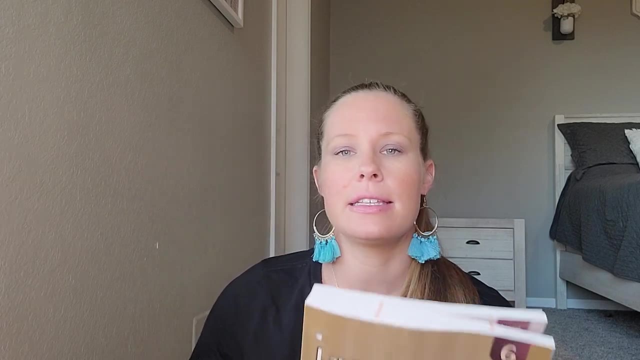 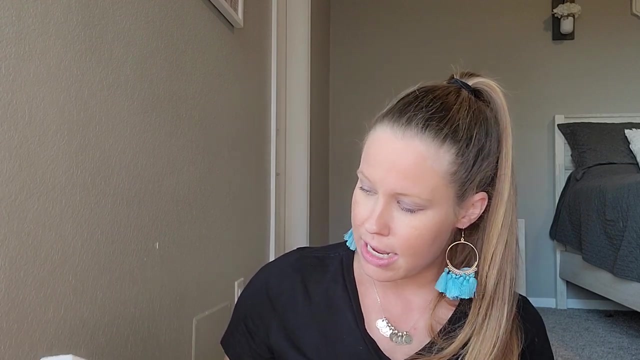 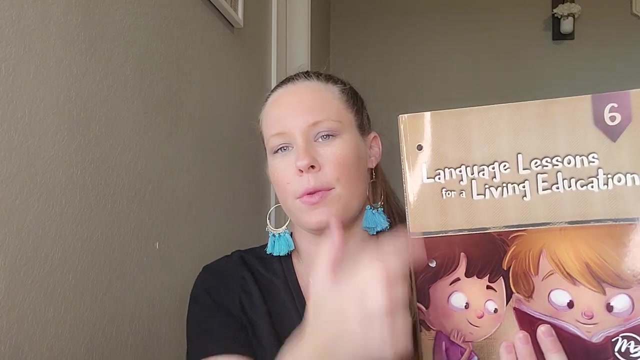 The thing that really struck out to me- stuck out to me, not struck out to me, stuck out to me- was the simplicity of these lessons. Um, at the beginning, let me take this up. at the beginning It talks about: um, these are also, they're books You can also put like in a three ring. 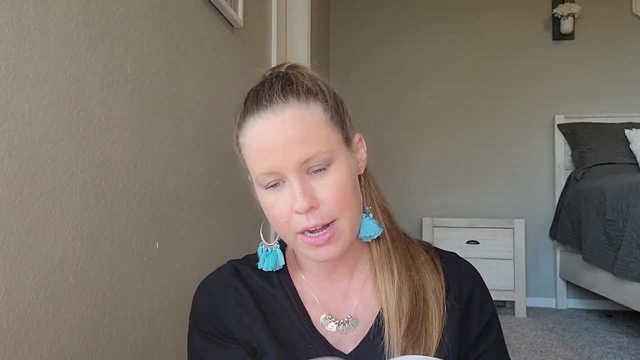 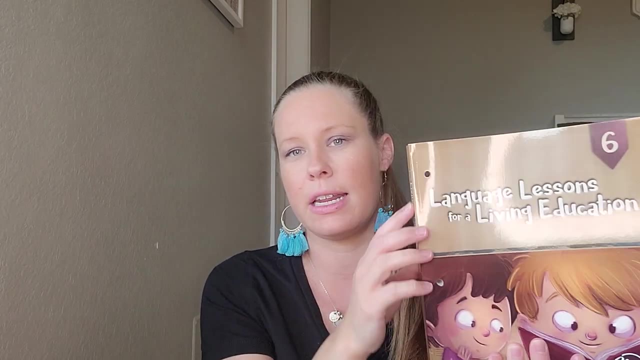 binder. that might be better, because these are like perforated pages. They might come out easily. So if that's something you want to do, I would maybe recommend that, sticking it in a binder and then you know the whole thing, and then, um, doing it that way. 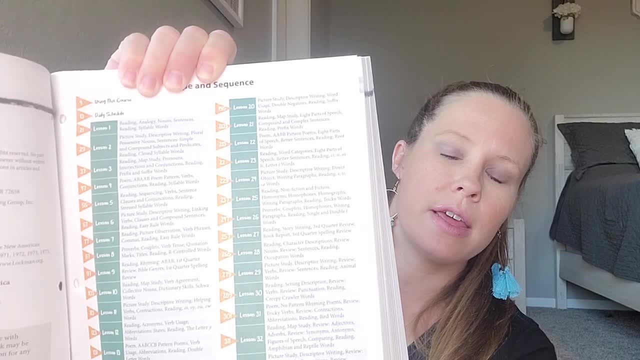 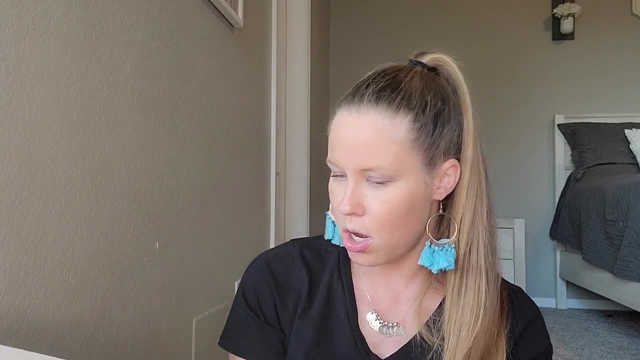 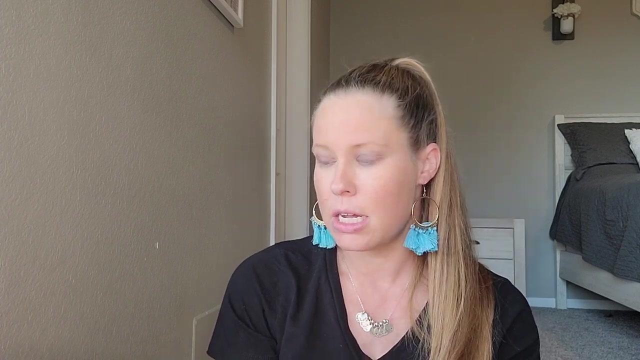 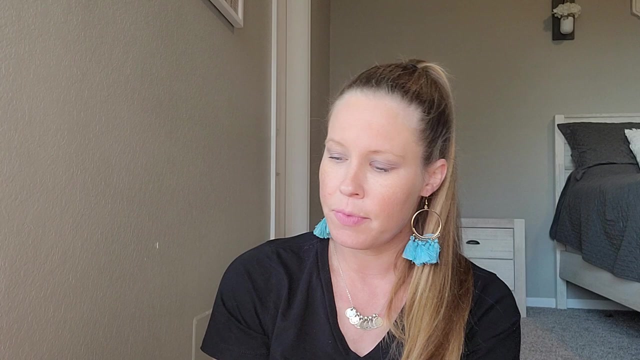 So you have your scope and sequence, So it will tell you everything. all the lessons there are: Do, do, do, do, do, do, do Um. there are 36 lessons, but um. within that, within those lessons there, you have multiple days, multiple things. 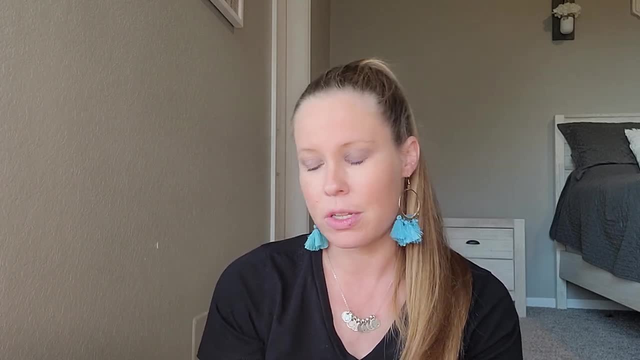 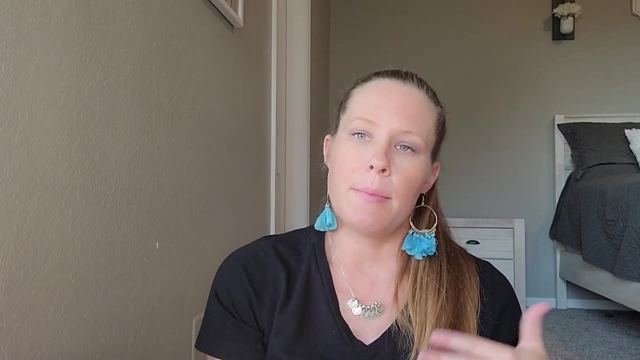 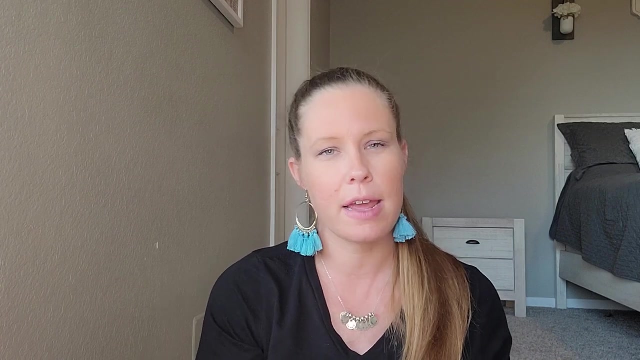 So, um, they will talk to you about the course description. They recommend approximately 20 to 30 minutes per lesson, five days a week. Um, we do five days a week Typically. um, my husband has off every other Friday and then is working from home on the other Fridays. 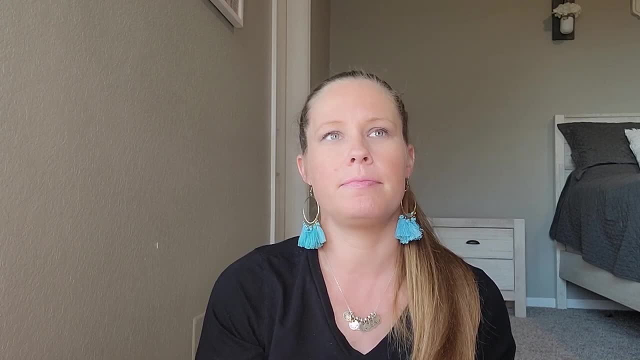 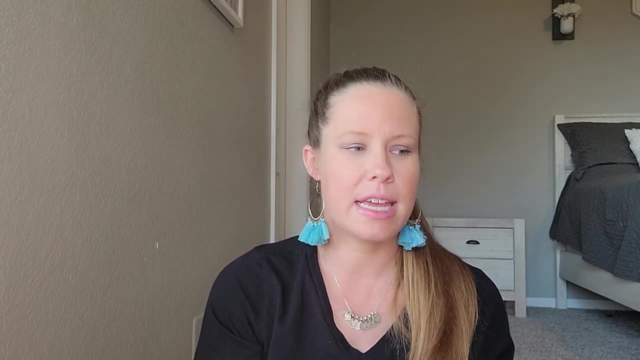 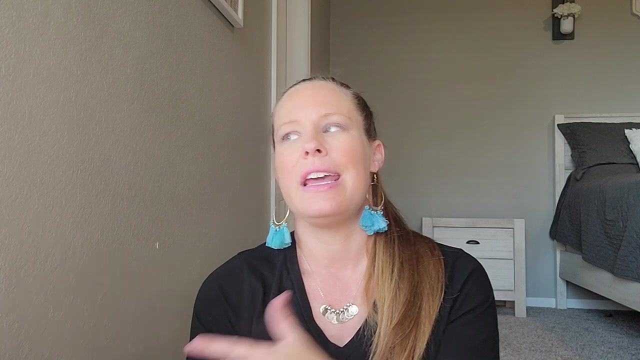 So I have thought about doing a four day week um curriculum or school week, but I think I just might kind of take it week by week. If he's working- obviously working from home, obviously my kids are going to be doing school- If he's not working that day, then maybe we'll go and just do something and just 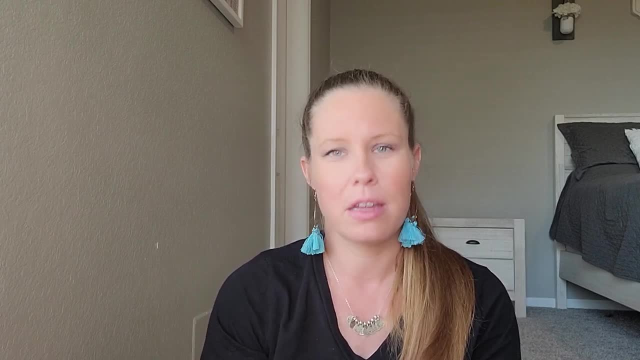 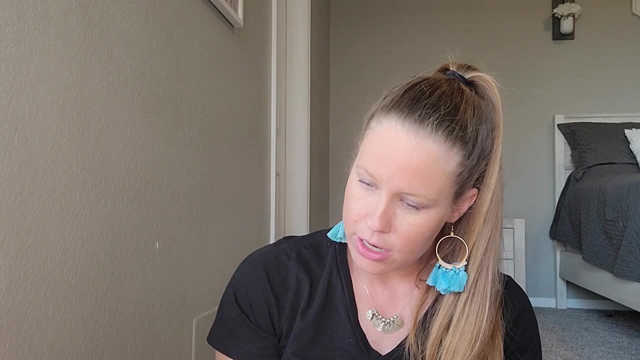 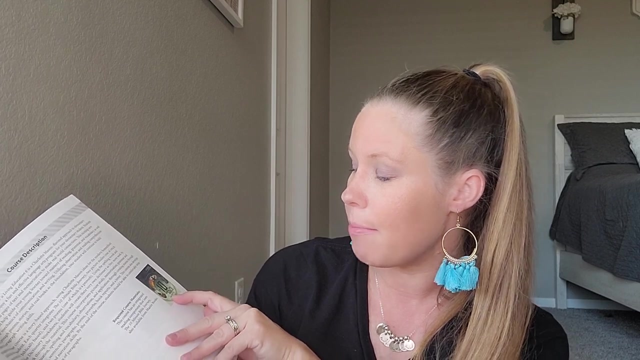 catch up later. Um, I don't necessarily want to make every week a four day week, So, um, um, let's see, this actually has a required course material. Um, it says this course has an integrated reading component that uses the 10 minute Bible journey, also available from: 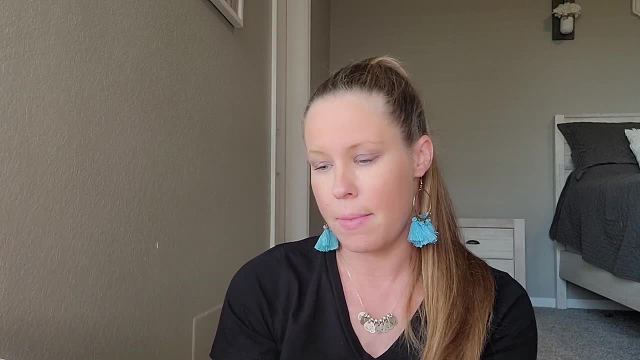 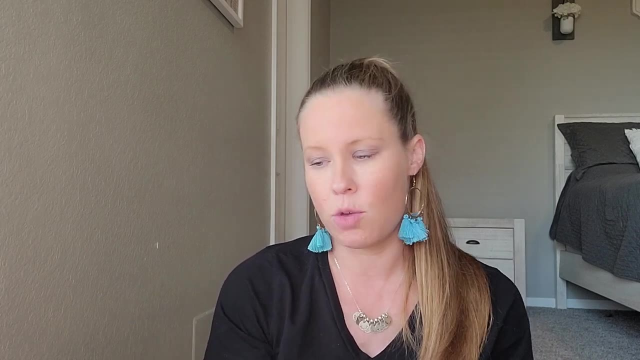 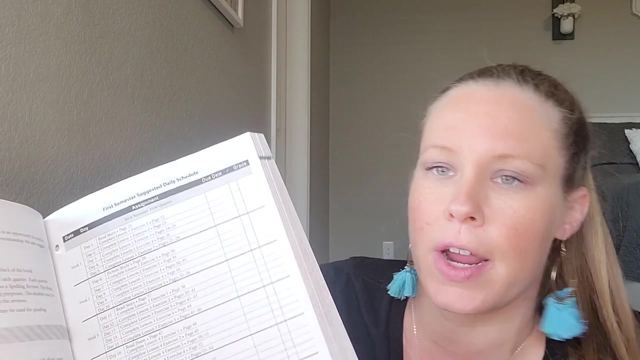 Masterbooks, So that is something that I need to get for them as well, for her as well. Um, it talks about all the different things that you will see in this curriculum. It has daily schedules, It has due dates, It has grades. We are not required in Texas to um record any grades whatsoever until high. 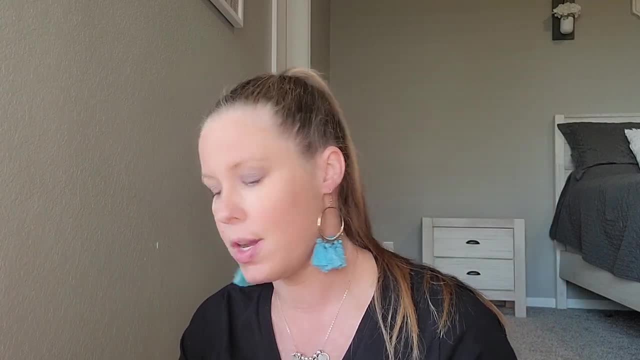 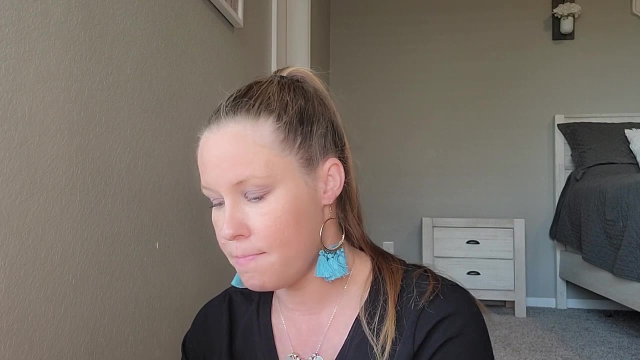 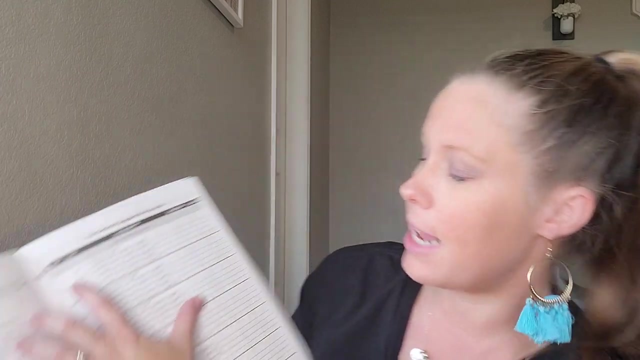 school obviously. So I do not do that for elementary, I do not do that for middle school. I will check things that need to be checked, But other than that I do not. um, I do not grade it, but at least it kind of has a layout for day one through five and kind of what to um do within. 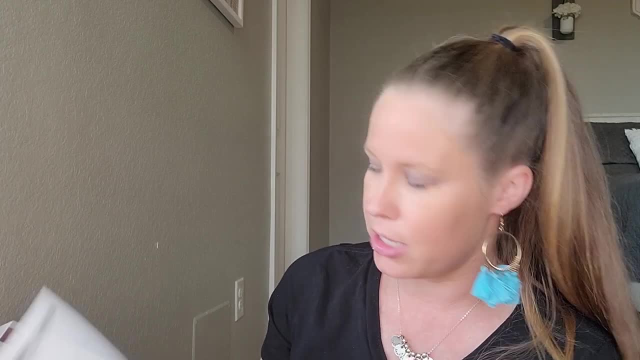 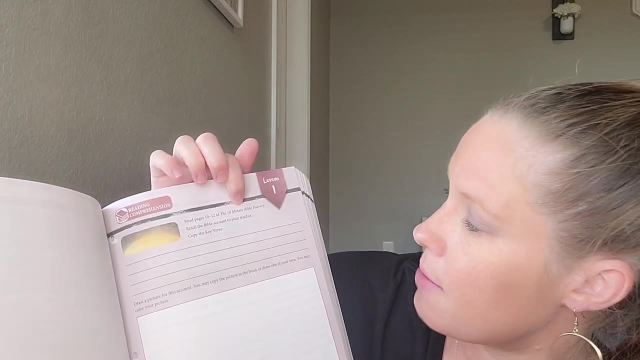 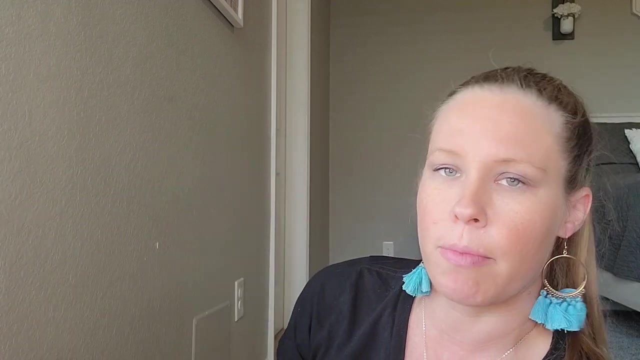 those, And then first semester and second semester. So, um, yeah, so even the very first lesson here has read pages 10 to 12 of the 10 minute Bible journey. retell the Bible account to your teacher, copy the verse, draw a picture. So it kind of has you know Bible stuff um integrated in here. 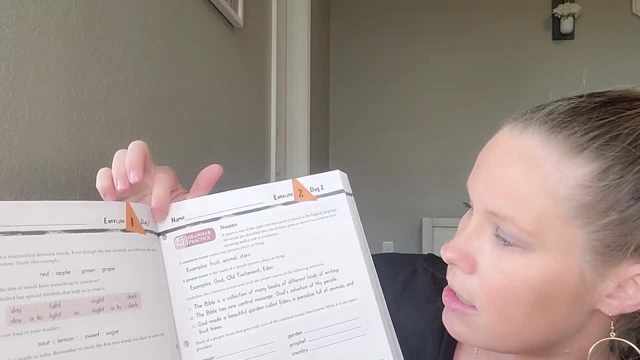 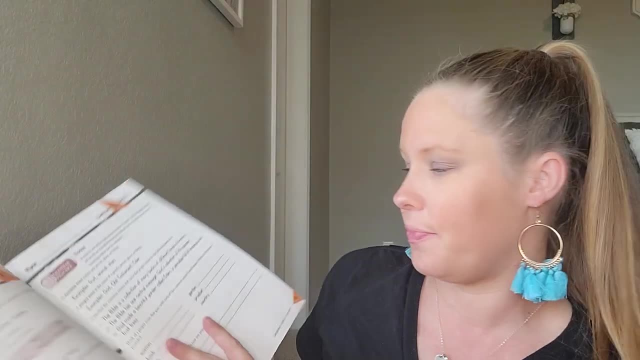 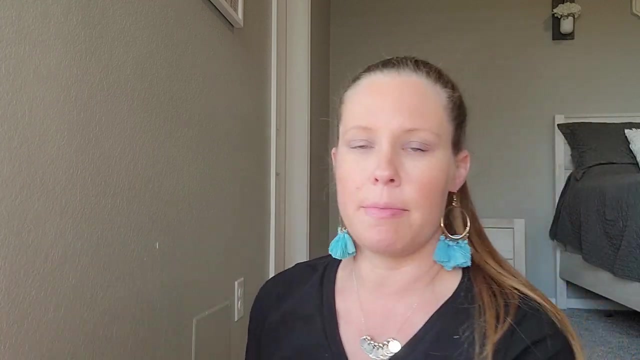 but it will start exercise one day one. So your lessons are so simple. They are so much easier. It's a lot easier than the good and the beautiful that we are used to Now. again, as in every curriculum piece, you are going to have refresher stuff at the beginning, So, while she might look, 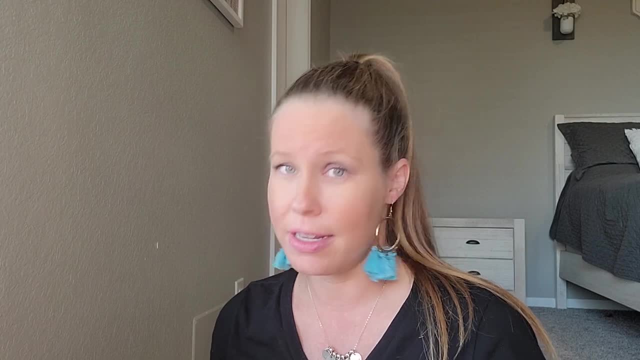 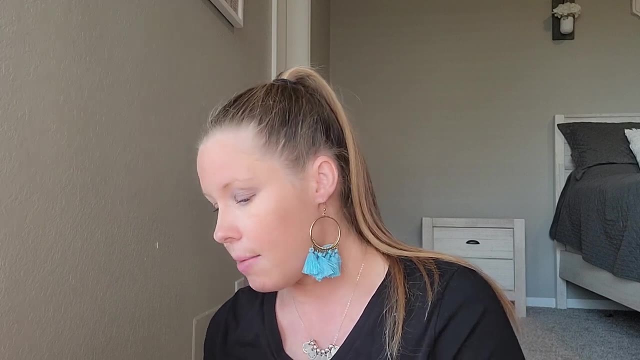 at this and be like: wait, I already know this stuff. Yes, you might, but I want you to keep going, because this is just to refresh your memory. Um, so, for example, there might be one page exercise one day, one. 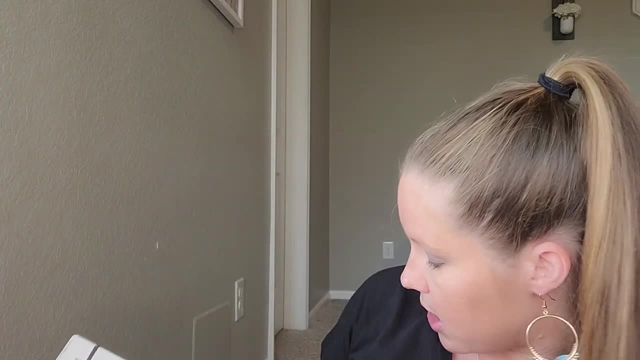 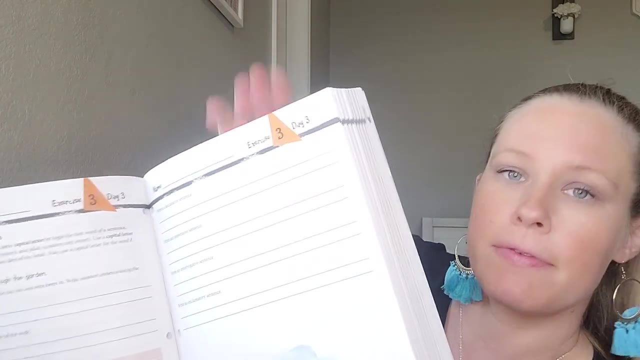 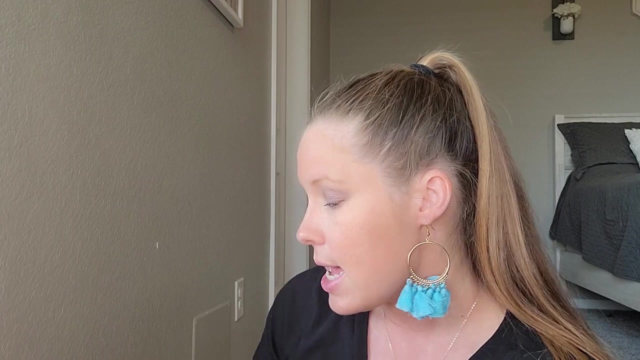 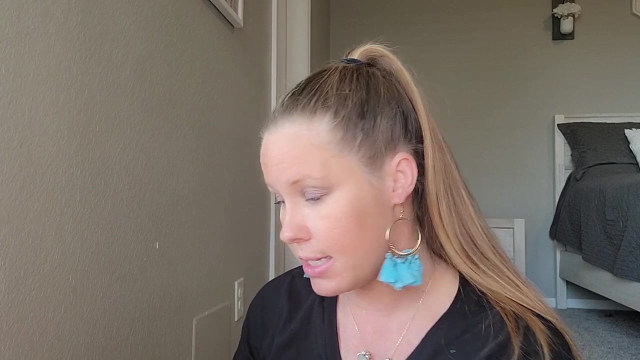 Exercise two, day two. exercise three: day three has two pages, So you just follow along: Um, so it will have the different kinds of sentences, It will have grammar practice. Um, it will have some writing. It will have, um, like I said, some reading comprehension. 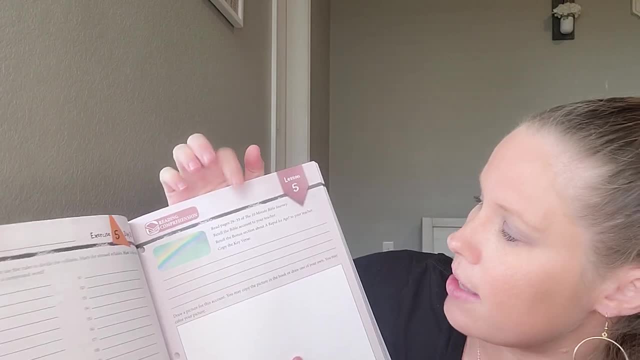 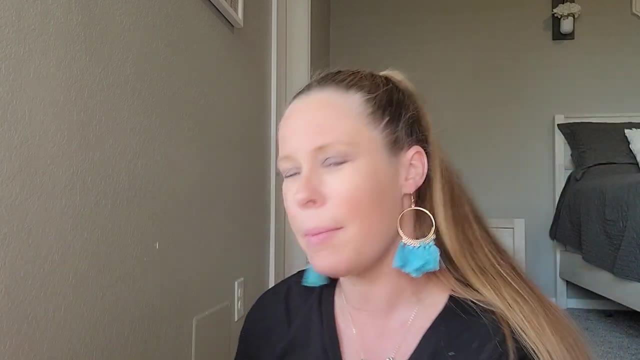 It looks like these grayish or brownish pages are the ones, um, that are in relation to the 10 minute Bible journey, So that one um, and that's kind of it, says: you know, retell the Bible account to your teacher. She likes to read the Bible to. 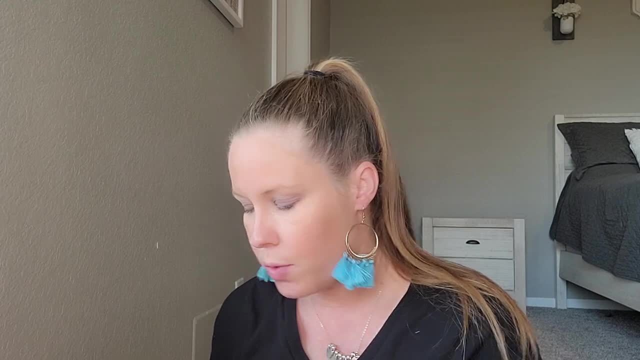 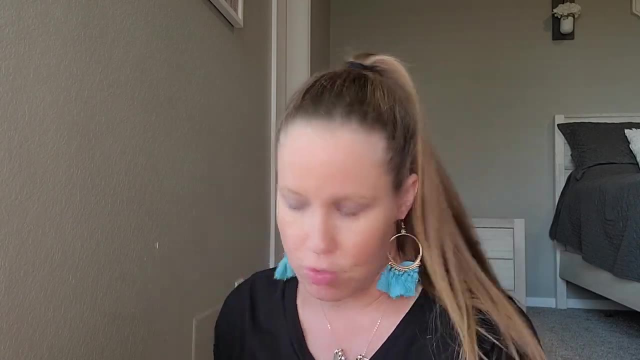 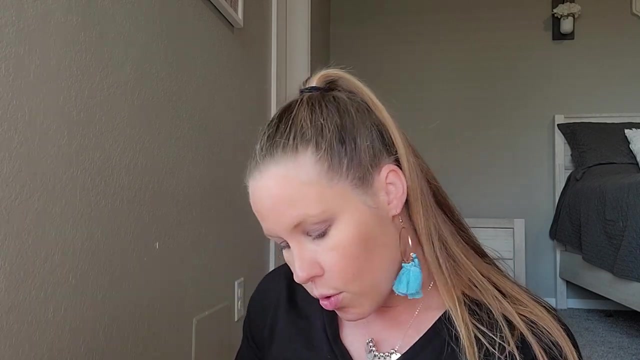 her younger siblings anyway, And so this is going to be. she's going to enjoy that. So if, um, you know, if you're not the Bible type or the religious type, don't do masterbooks, because it's it's going to be. um has a religious aspect to it, Um syllables. 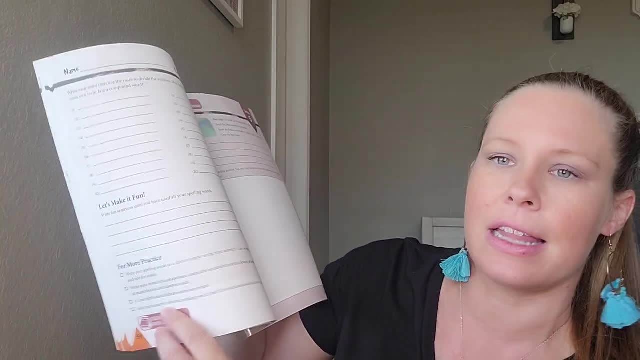 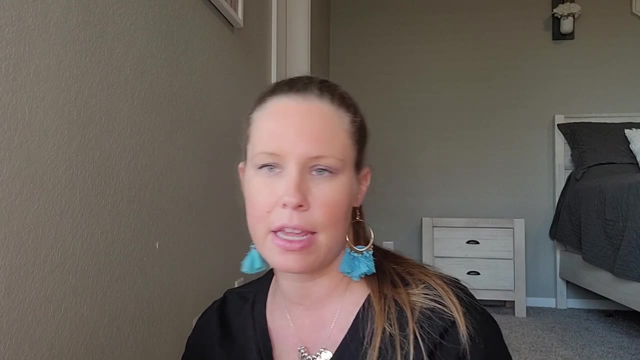 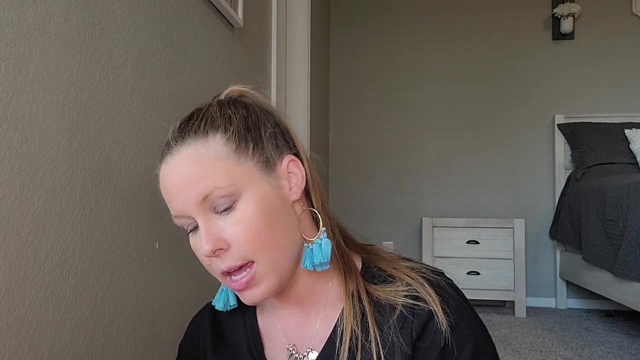 for more practice it has down here. That's something that, like I, will take lesson by lesson or whenever I see it and determine whether or not that's something that I think she would enjoy doing. Um, but that is pretty much how it's laid out. I um, they have like map studies here. 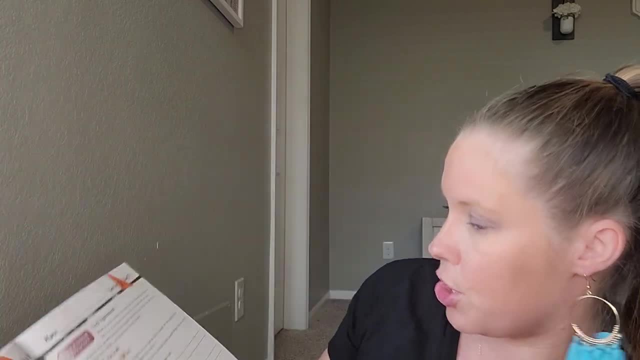 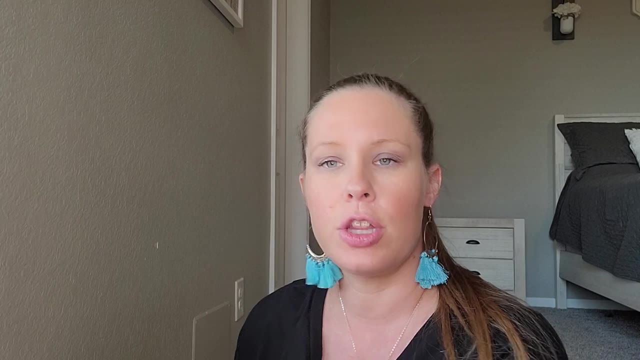 Um, they have independent reading that they'll want you to do And that can be, you know, from whatever reading you want to do If you want to get. I like the good and the beautiful book lists that they have, because you know those are. 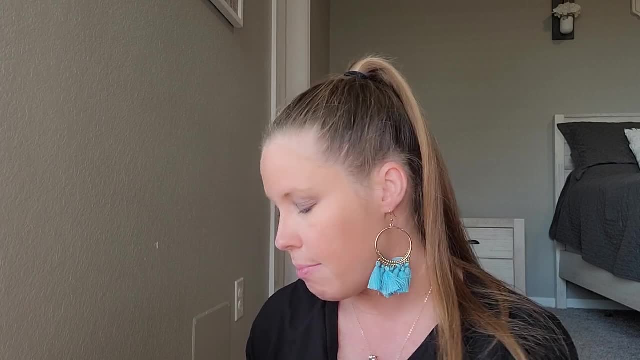 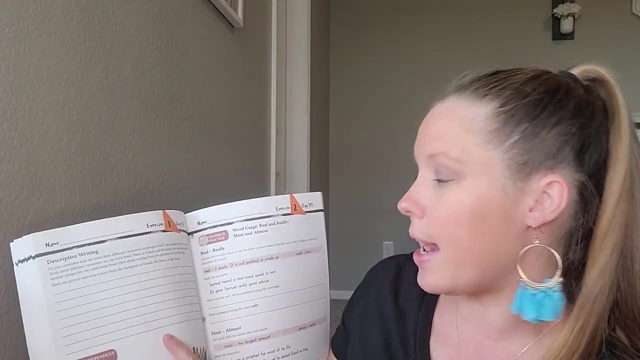 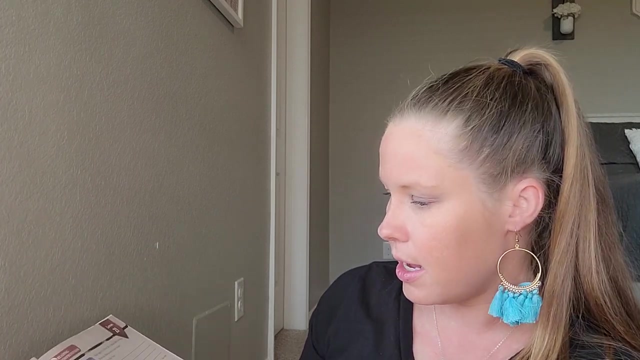 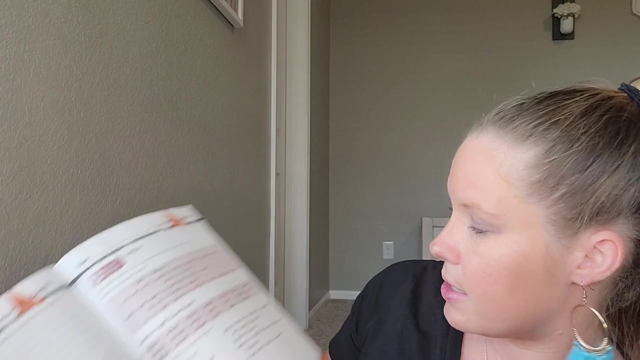 clean um books, but you can have them read from wherever um descriptive writing, So you will have writing pieces here Um, you will have. let's see, I think it has okay, So here's like there is some spelling integrated in here as well. So spelling practice, So they will have. 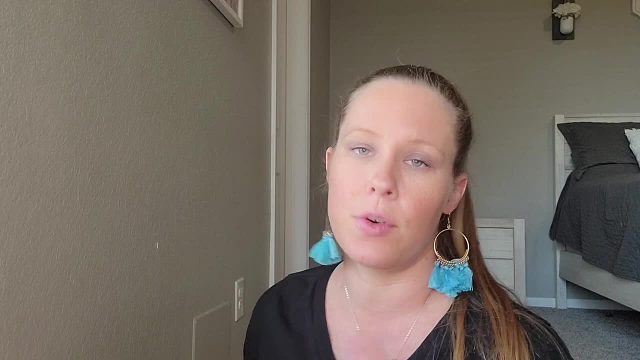 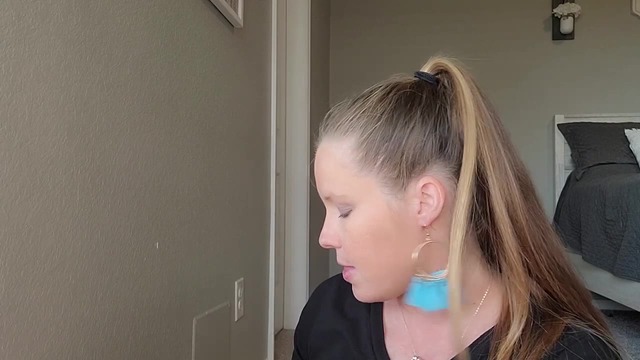 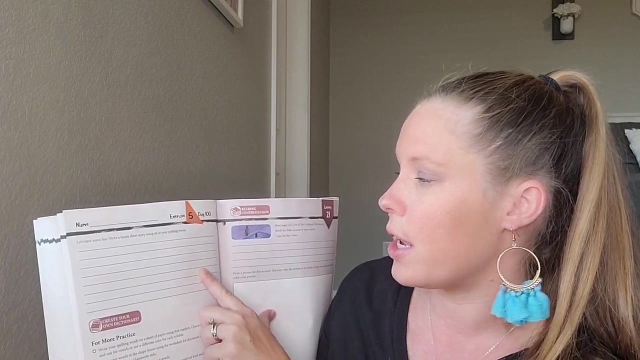 spelling, learn how to spell these words. So she is also doing a spelling curriculum. but this is these. these lessons are so short. Why not just do them Um, and I think it's good practice for any way. So the little writing um blurb here would be um write a funny story. 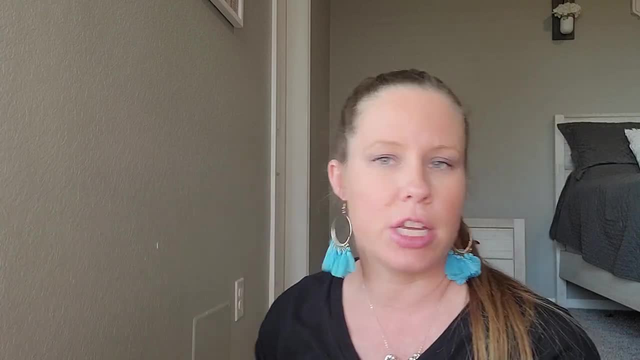 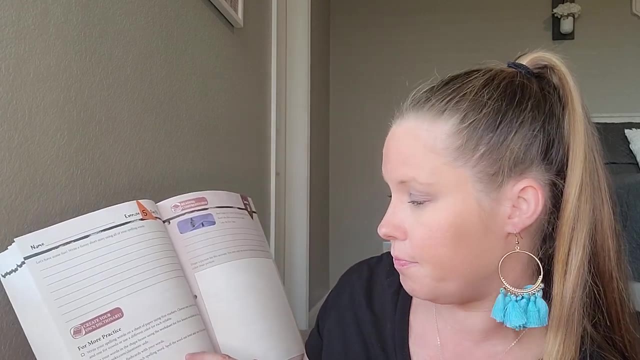 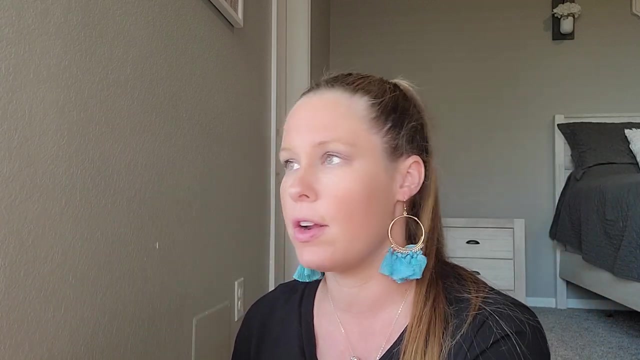 funny short story using all of your spelling words. So that's something that she can do if she wants. if not, totally fine. Um, for more practice, you have, um, you know little things here. that if you have time, great. If not, I'm one of those people that, if there is, 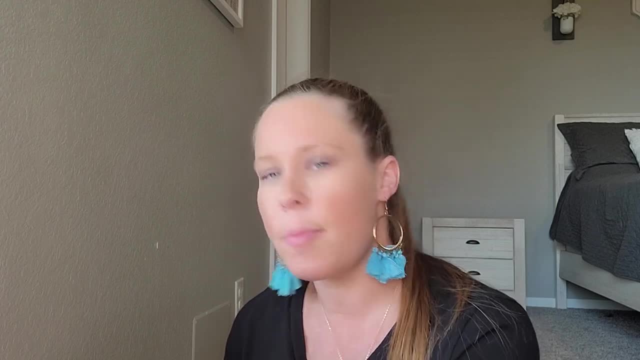 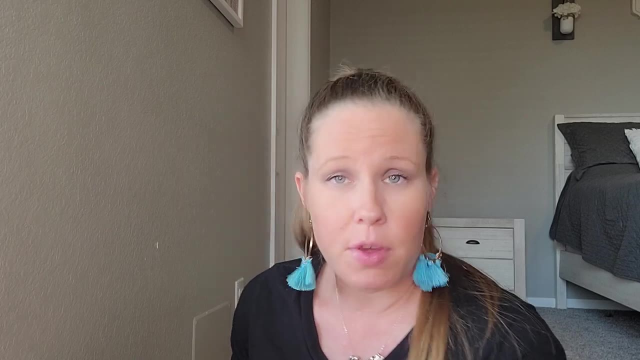 extra stuff in the curriculum, extra stuff that's optional. I give them that option. Do you want to do it? Yes, Do you have time to do it? Do you have extra time? Do you have? go ahead and do it if you. 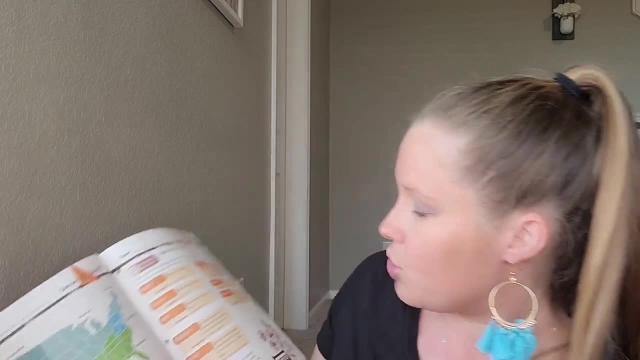 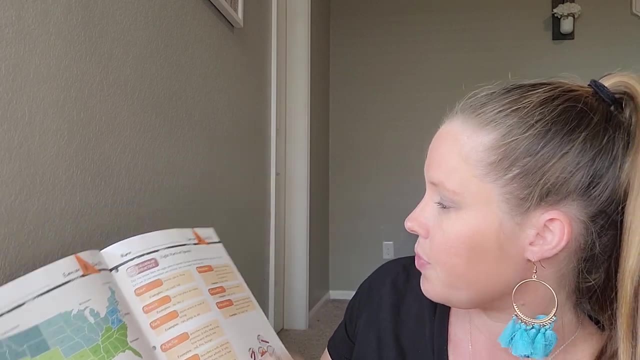 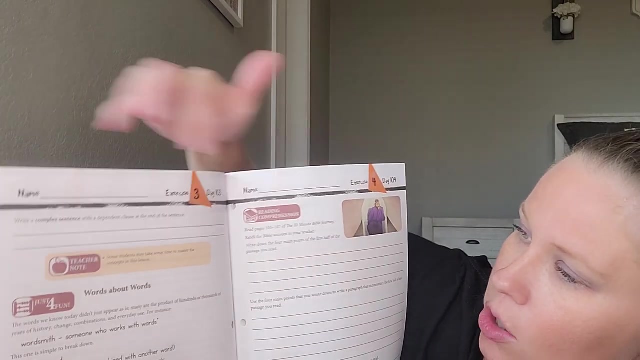 want, if not, move past it. Um, it does have some geography in here. So the different States separated, I mean the different parts of the United States separated, the parts of speech it has, And it'll show at you know on each lesson what it's actually for. So just for fun reading, 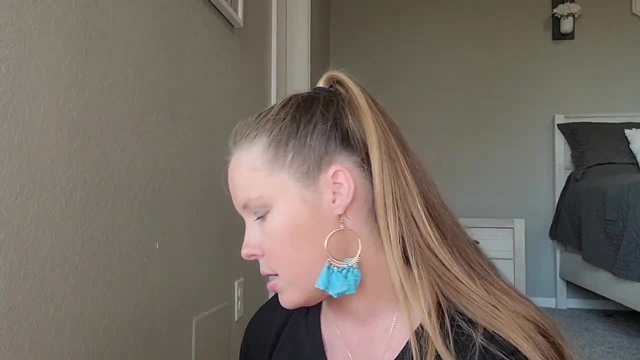 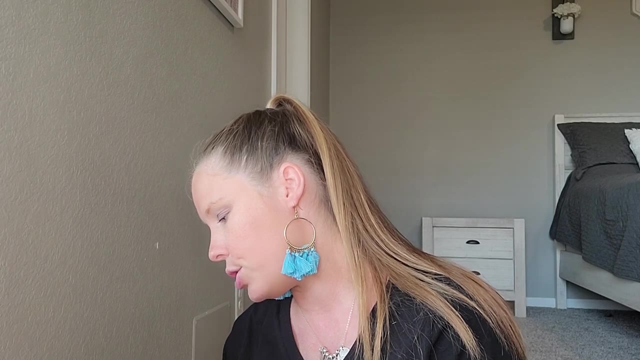 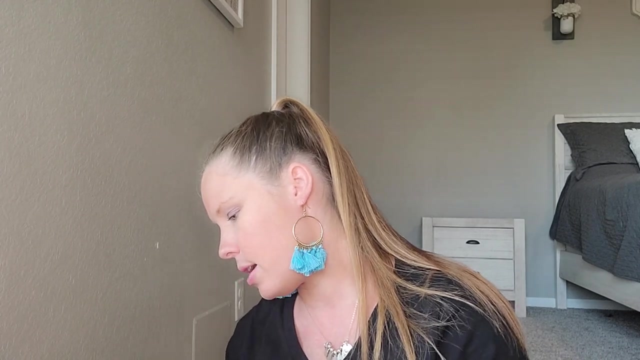 comprehension and, um, you know, your spelling practice, all of that. So this has, let's see, it goes all the way to: uh, let's see, day, What did I say? Day, This goes to day. 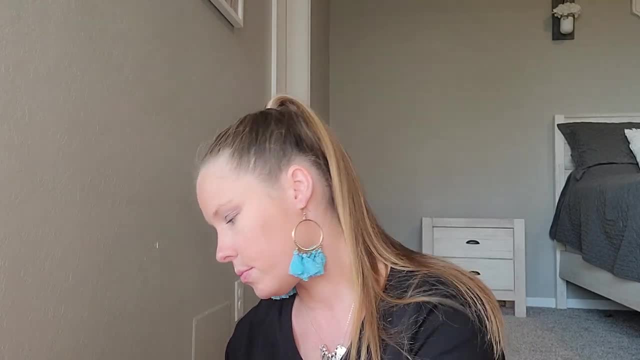 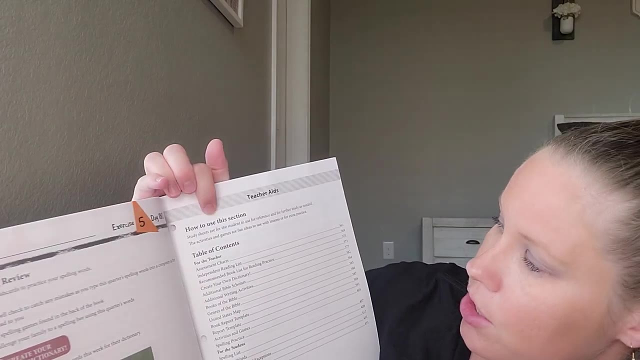 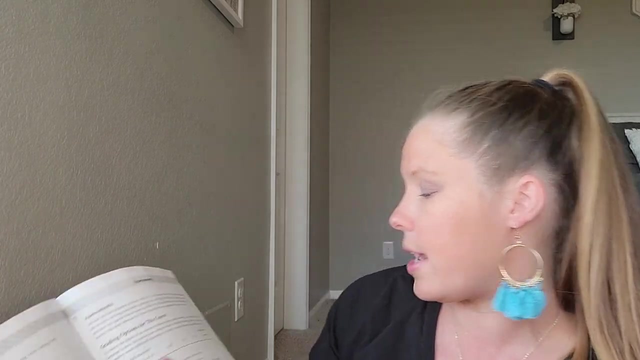 Uh, one 80. Yes, Day one 80.. Um, so in the back of the book it has it shows you your teacher aid. So this is kind of for your own reference here. It has um grading If you want to do. 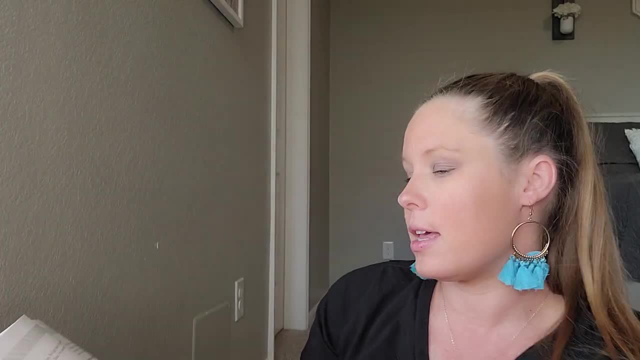 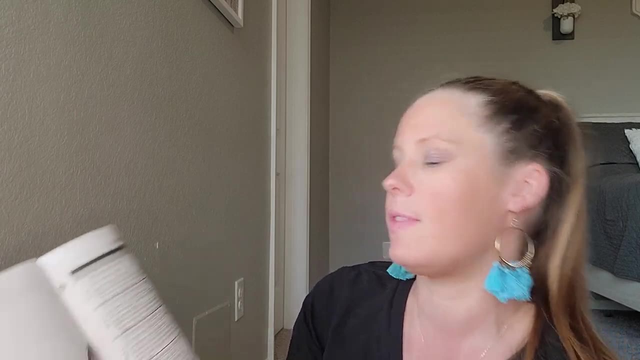 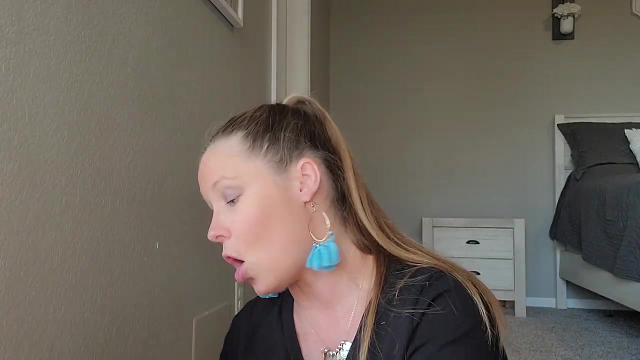 grading. it has how to grade the um assignments. It has. you know, if you want, like I said, these a lot of this is maybe for people in States where they require these kinds of things, Um, and this kind of log. 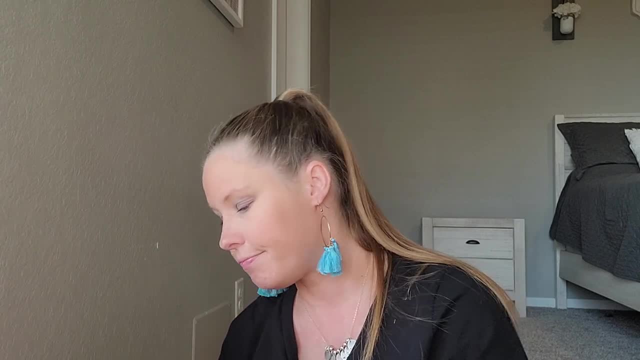 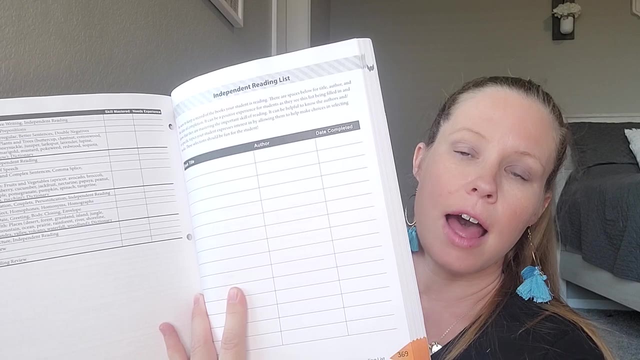 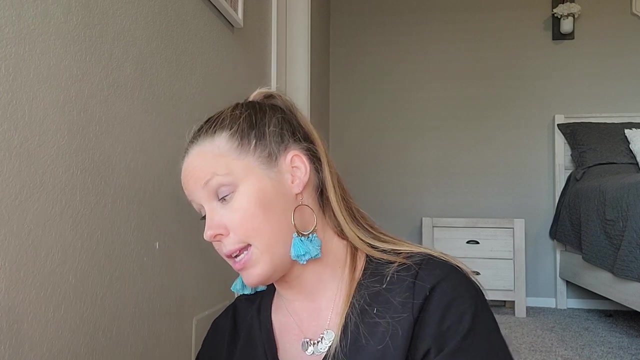 skills mastered, whether it needs needs, um needs help. They need help with certain things. independent reading list: If you wanted to keep a list of all of their independent reading, for whatever reason, So here are. actually they have a recommended book list for reading practice. 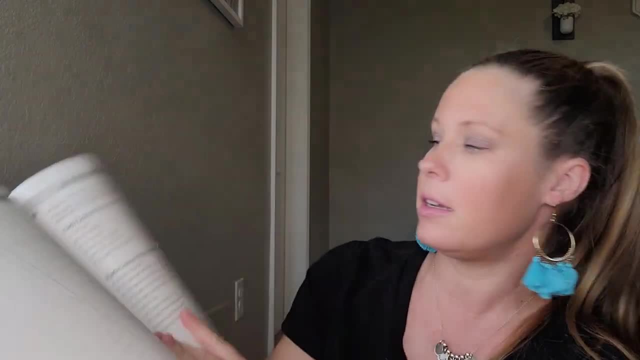 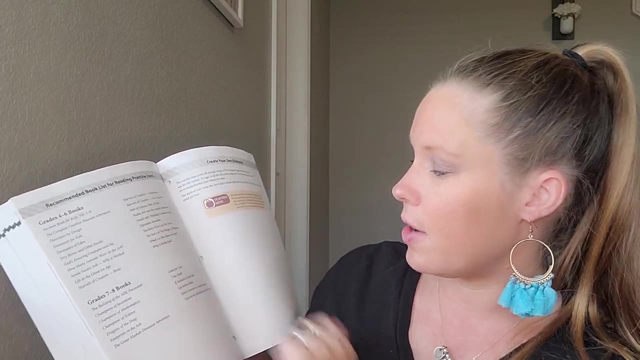 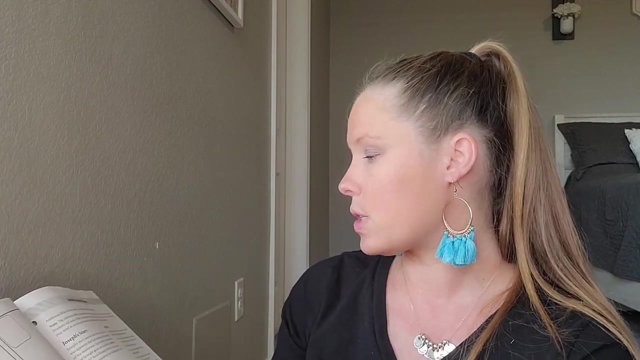 separated into grades, which is nice. I didn't know they had that. So early learner, uh, grades K through three, grades four through six and grades seven through eight. So that's neat. Um, and then they have additional- let's see additional- Bible scholars. 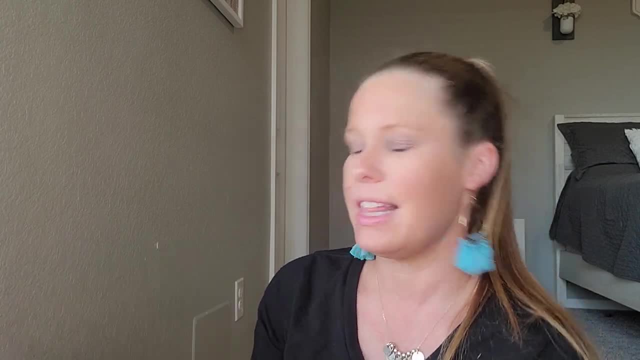 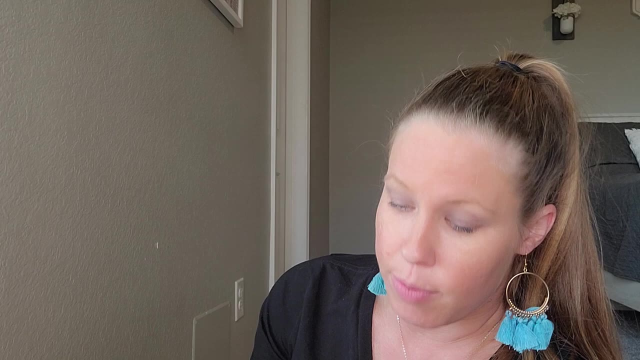 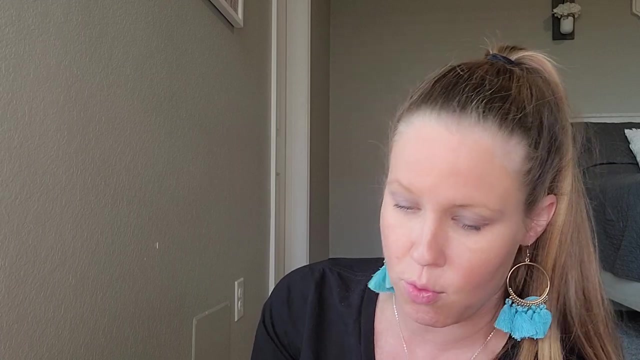 They may be assigned for more study opportunities. That's kind of just extra stuff. Um, they have additional writing activities, the books of the Bible, the genres of the Bible, the map, the um book report template- If you wanted to do a book report um activities and games they have. um, where did I see the other?